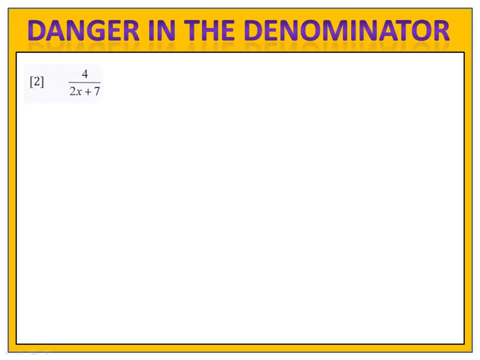 a variable down there. There are certain numbers we cannot plug in for x because that will cause us to have 4 over zero. 2x plus 7 cannot equal zero or we have a zero in the denominator. That's a big problem. We solve that little piece: 2x plus 7 equals zero and we see that. 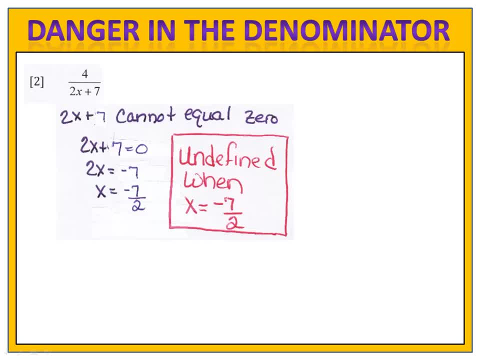 x equals negative 7 halves is the problem. This fraction is undefined when x equals negative 7 halves. In other words, if we took the fraction and plugged in negative 7 halves, we'd end up with 4 over zero, and we can never divide by zero. So the value for which this fraction 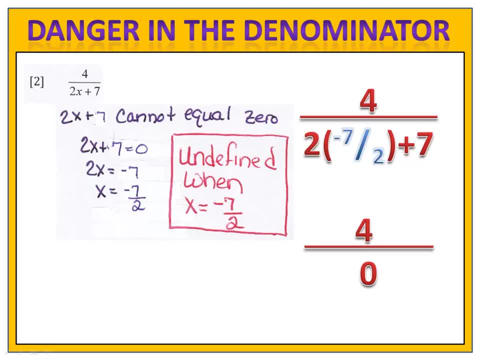 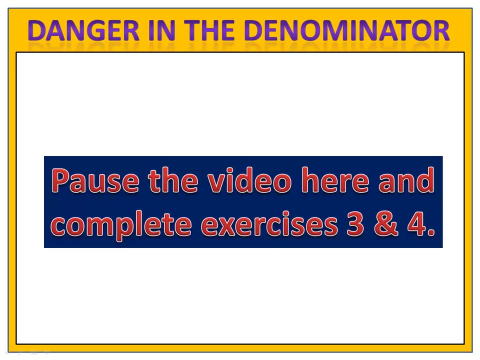 is undefined is negative. 7 halves In exercise 3 and 4, these are for you to. to try, Please see if you can find the value that causes danger in the denominator. Please pause the video here and complete exercises 3 and 4.. 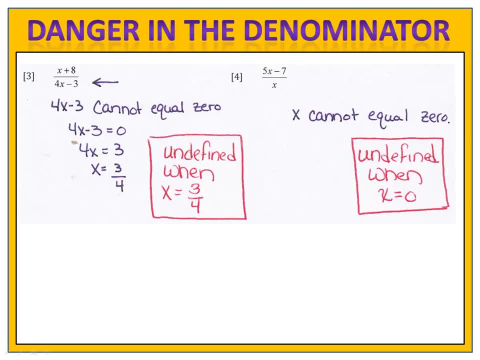 In exercise 3, we see there's danger in the denominator, because 4x minus 3 cannot equal 0. We find the value that would cause that to equal 0 and we get x is 3 fourths. In other words, if we put the number 3 fourths in for x, we have a fraction with 0 in the 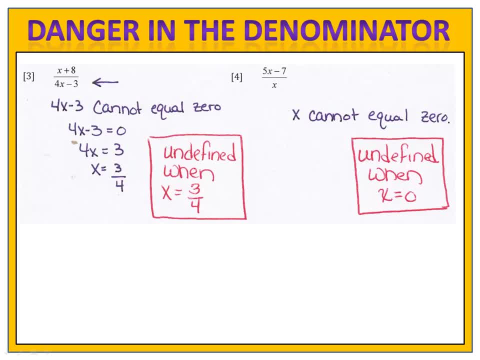 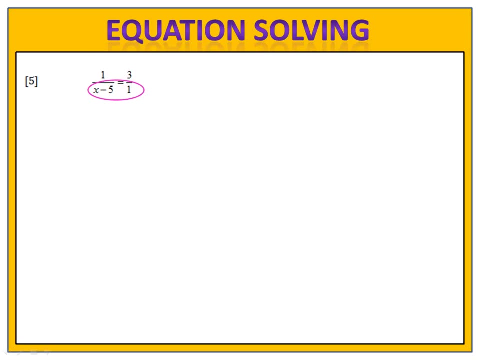 denominator. In example 4, x cannot be 0. If x is 0, we have something over 0 and we cannot have the denominator equal to 0.. Now let's talk about equation solving. In exercise 5, we have an equation because we 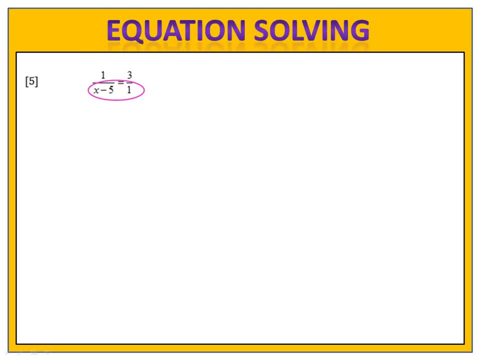 have two things equal to one another. We need to begin by clearing our denominator. We'll begin by clearing our denominator. We'll begin by clearing our denominator. We'll begin by multiplying both sides by x minus 5.. This causes the x minus 5s on the left hand side. 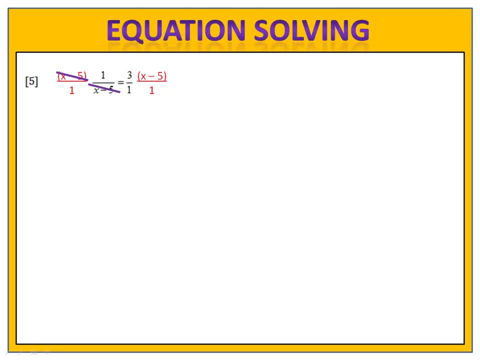 to cancel out, and now there are no variables left in the denominator. We now have 1 equals 3 times x minus 5.. We know how to solve that equation using the properties of equality and we get x equals 16 over 3.. It's really important to check your answer when you get. 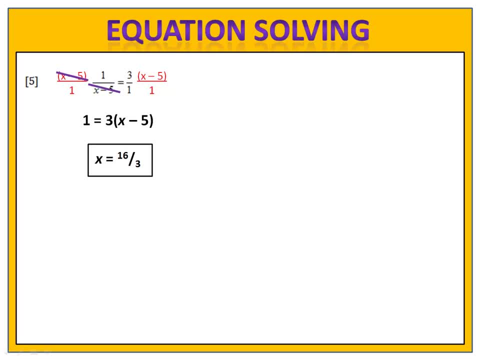 your value for the equation to make sure that it doesn't cause a 0 in the denominator. 16 thirds does not, and so the answer x equals 16 thirds is our solution to the equation In exercise 6,. we're going to do something very similar Here. notice we have a variable. 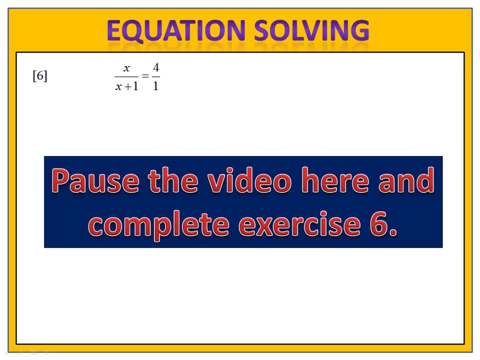 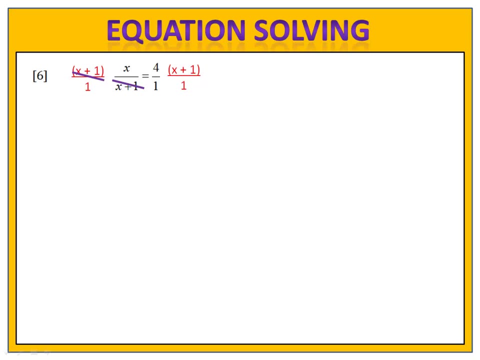 in the denominator x plus 1.. Please pause the video here and complete exercise 6.. We begin by multiplying both sides of the equation by x plus 1.. We'll begin by multiplying both sides of the equation by x plus 1.. This causes the x plus 1s to cancel out. and now? 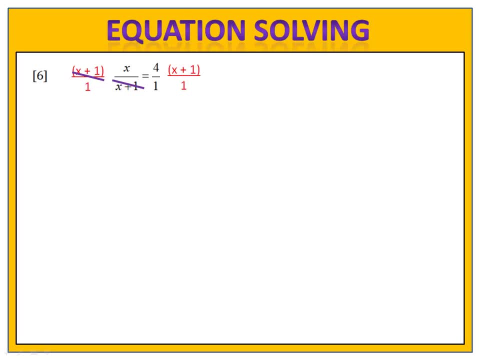 I have no more variables left in the denominator and I can solve this equation. I have: x equals 4 times x plus 1, which means x equals negative 4 thirds. Again, remember to check your answer and plug it into the original equation, Be sure it doesn't cause danger in the denominator. 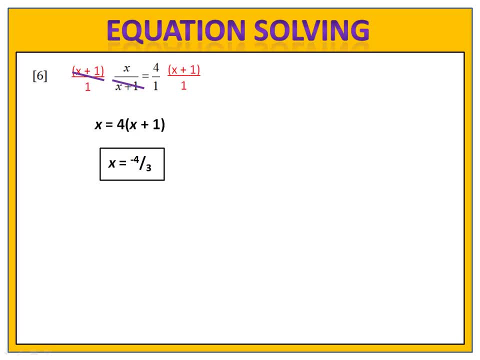 by causing it to be 0 in the bottom of the fraction. In this case it does not. so the solution x equals negative 4 thirds is our solution to the equation. We're going to do something very similar here. In this example, y equals minus 2 where x equals negative. 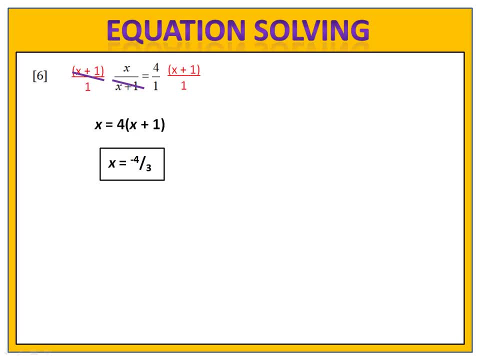 4 thirds is our set of highlighted values and x equals y equals negative. 4 thirds is valid and that's our solution to the equation. In exercise 7, we have 7 over p minus 6 equals 17 over p minus 17.. Please pause the video here and complete exercise 7.. In this exercise, 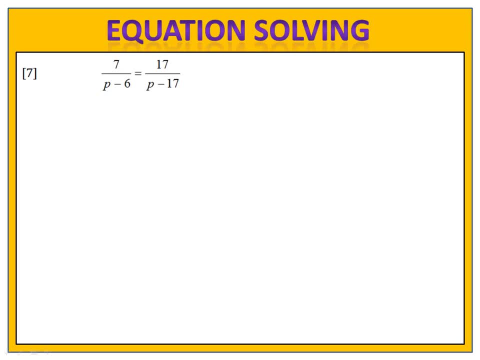 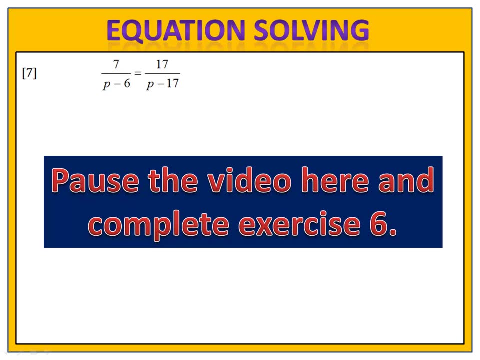 we begin by multiplying both sides by p minus 6.. That causes the p minus 6 on the left-hand side to be 0. The problem here is not that we only miscalculated by 1. We obtained here the result that p plus 4 is printed and 1 and x equals 17.. Here observe how Iκmultiply. 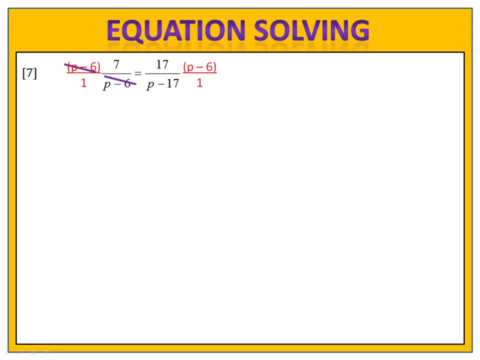 to cancel out. and now we have to deal with the p minus 17 on the other side. If we multiply both sides of the equation by p minus 17, those cancel out on the right hand side, and now I have no more denominators to worry about, so I can solve the equation. I have p minus 17 times 7 equals 17. 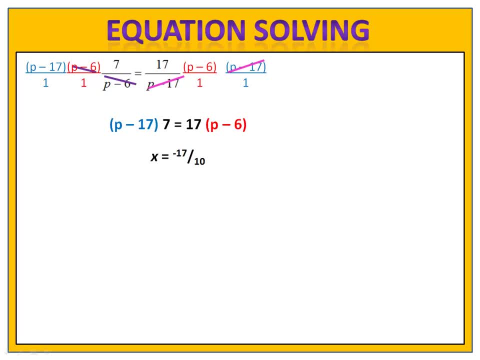 times p minus 6.. I can use the distributive property to solve the equation and I get x equals negative 17 over 10.. Remember to check that solution in the original equation, the equation that's printed on the page Here. negative 17 over 10 does not cause any problems because it doesn't.